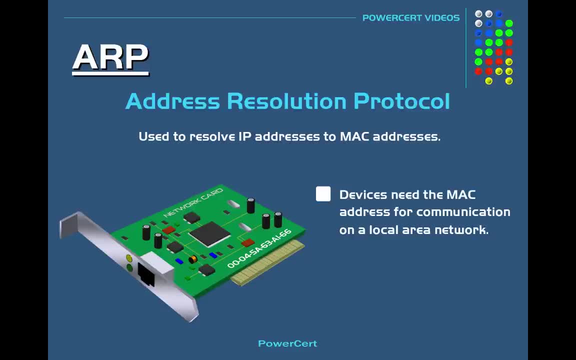 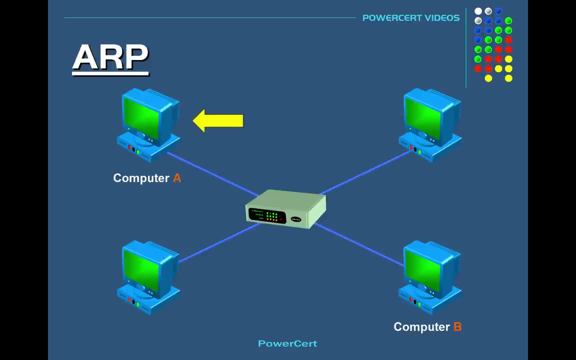 communicate with another device on a local area network, it needs the MAC address for that device, And devices use ARP to acquire the MAC address for that device. So as an example, let's say that computer A wants to communicate with computer B. Now computer A. 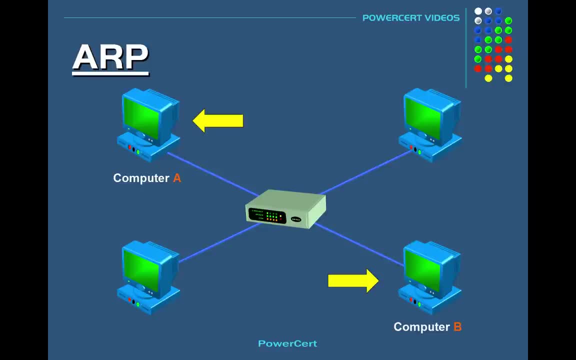 already knows the IP address for computer B, But in order to communicate with computer B, it still needs its MAC address. Now, an IP address is used to locate a device on a network, And the MAC address is what identifies the actual device. So, in order to find the MAC address, 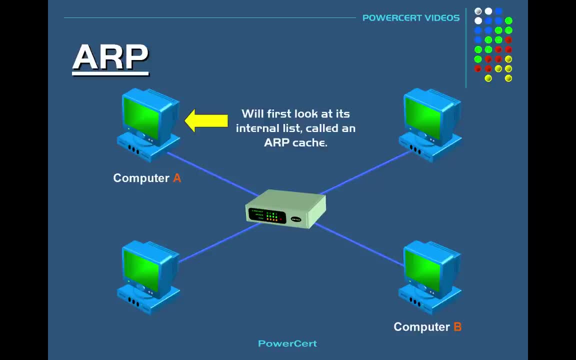 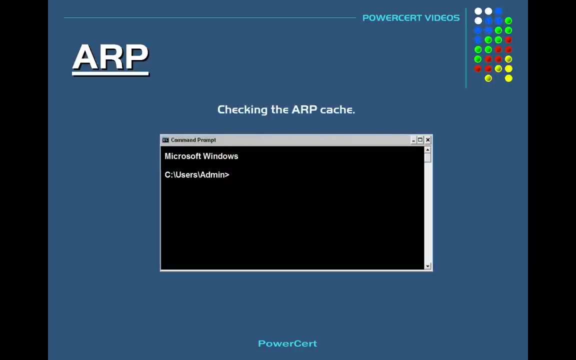 computer A will first look at its internal list, called an ARP cache, to see if computer B's IP address already has a matching MAC address. In fact, we can check this ourselves at a Windows command prompt by using the ARP utility and by typing ARP space. 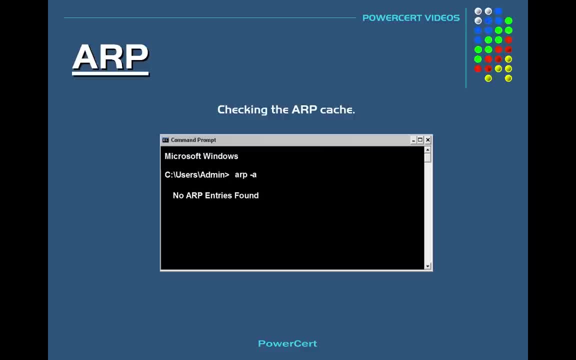 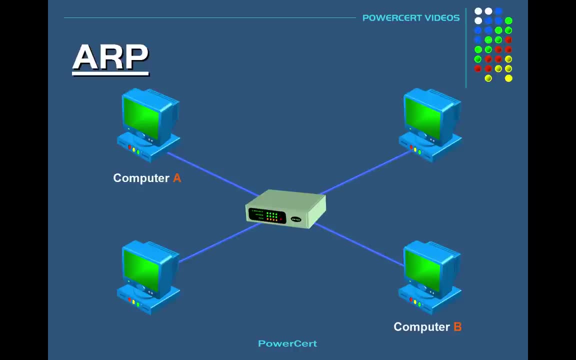 And as you can see in the output, it has no entries at all. The ARP cache is empty. So now computer A will send out a broadcast message out on the network asking every device which computer has the specific IP address and will ask for their MAC address. Then the computer 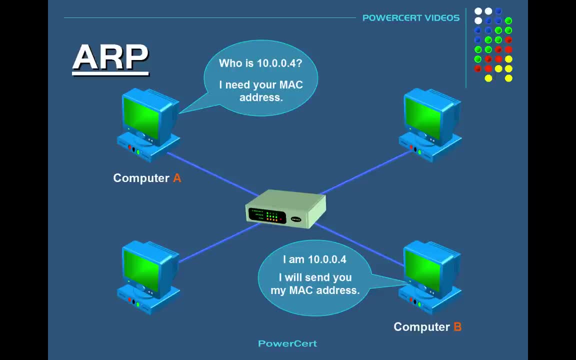 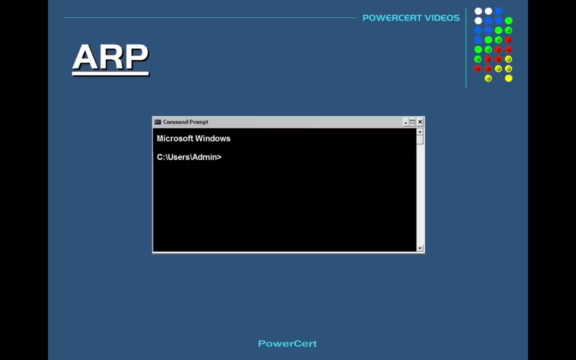 that has the matching IP address will then respond back and tell computer A its MAC address. Then, once it receives the MAC address, the communication can now take place between the two. Now, once computer A has the MAC address, it'll store this information in the ARP cache. 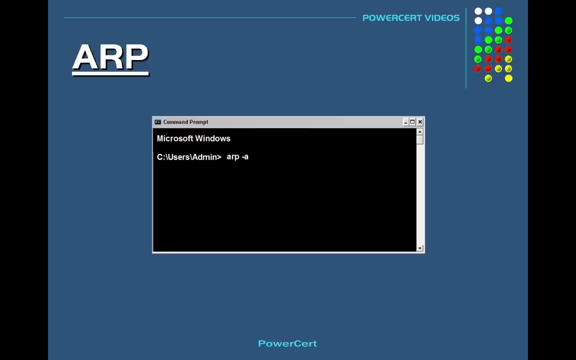 So now let's do the same commands as before, And now you can see that the IP address and matching MAC address have been added to the ARP cache. The ARP cache is used to make a network efficient. It stores IP address to MAC address associations so that the next time it needs to.